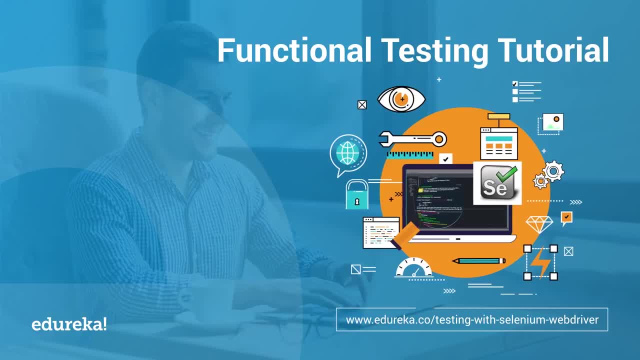 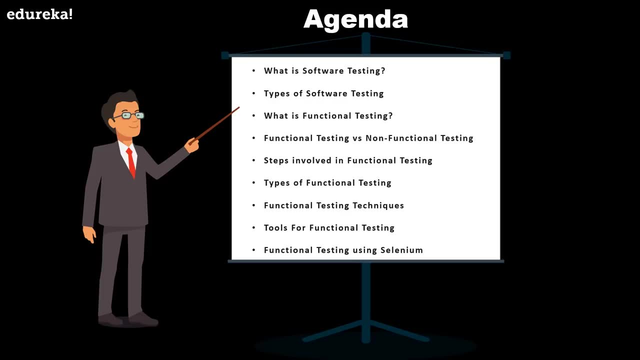 functional testing. now, before we begin with our functional testing tutorial, Let's have a look at today's agenda. So first I'll tell you what is software testing and then we will move on and have a look at the types of software testing. then we will discuss about what is functional testing. 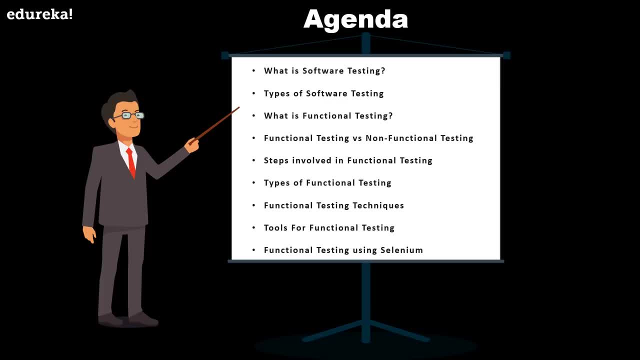 and also the difference between functional testing and non-functional testing. next up, We will have a look at all the steps involved in functional testing, and then we will have a look at all the different types of this testing. now moving on, We will also have a look at the different techniques involved. 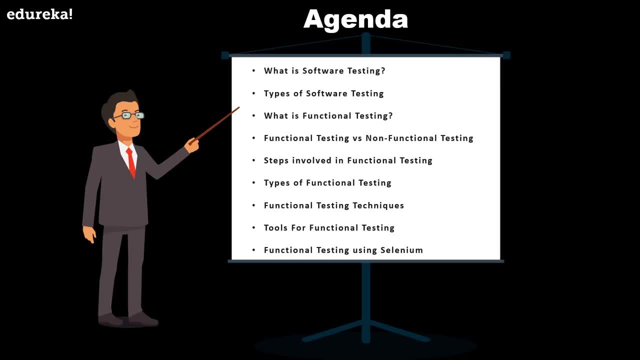 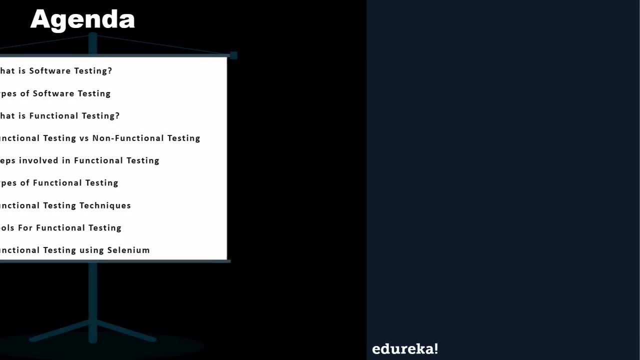 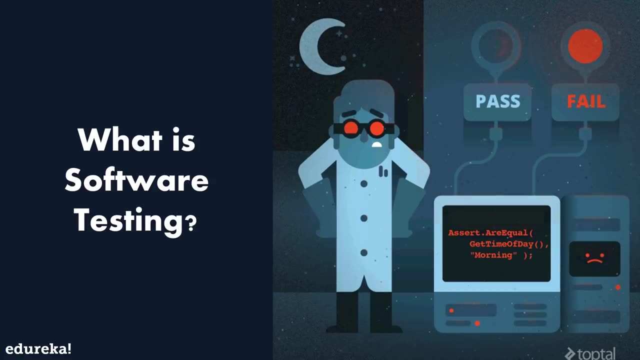 in functional testing and the tools that are used. Finally, I'll end this session with an example of how we use the selenium tool in order to perform functional testing. So let's get started now. software testing is a process of evaluating the functionality of a software application, to find 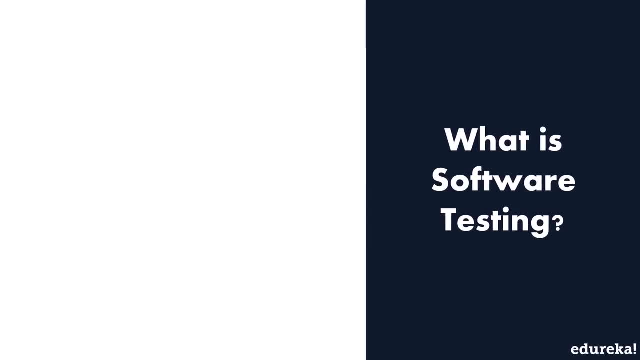 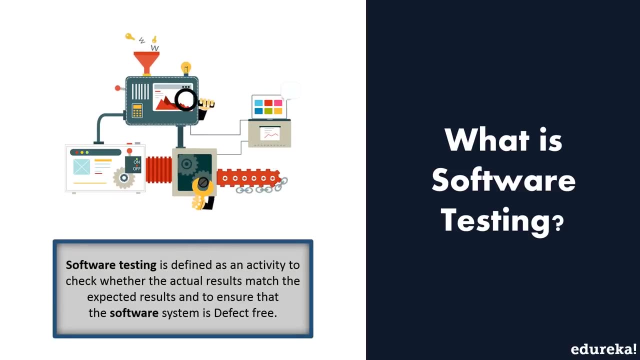 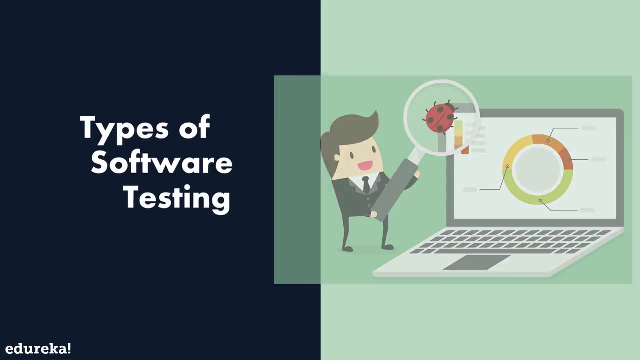 any software Bugs. it basically checks whether the developed software met the specified requirements or not and identifies any defect in the software in order to produce a quality product. Now let's have a look at the different types of software testing. So software testing is basically divided into two. 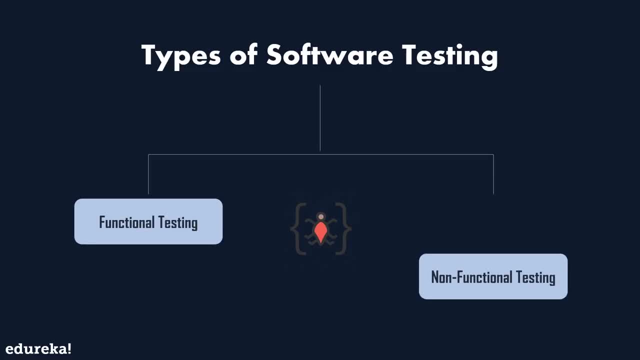 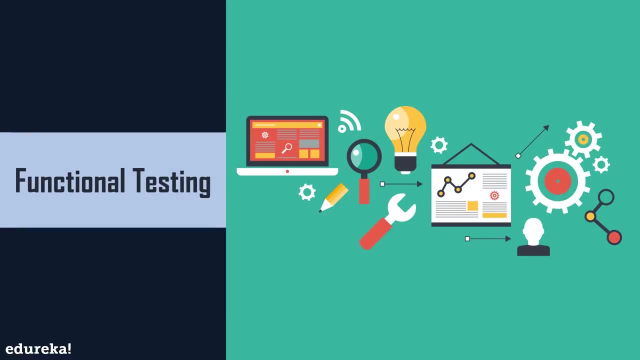 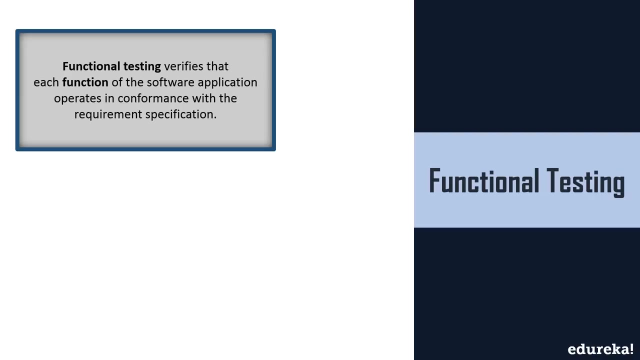 major types, that is, the functional testing and non-functional testing, and for today's session, Our focus will be on the functional testing type. So what is functional testing now? this particular testing is defined as a type of testing which verifies that each function of the software application operates in conformance with the requirements. 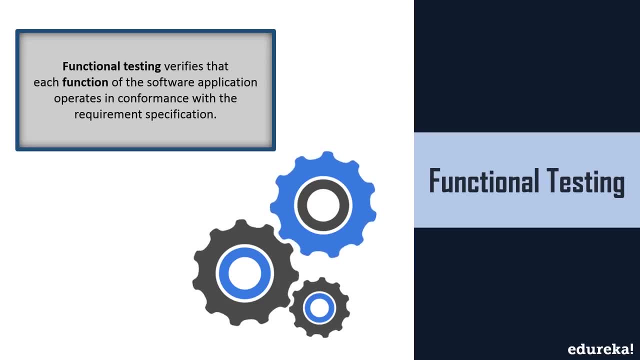 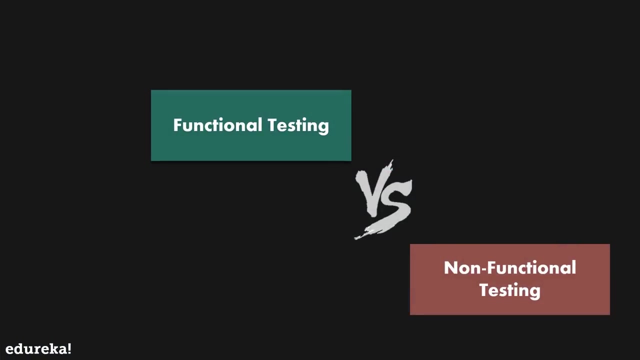 specification. now, this testing mainly involves the black box testing and it is not concerned about the source code of the application. now, each and every functionality of the system is tested by providing appropriate input, verifying the output and comparing the actual results with the expected results. So now let's have a look at the differences between functional testing and non-functional testing. 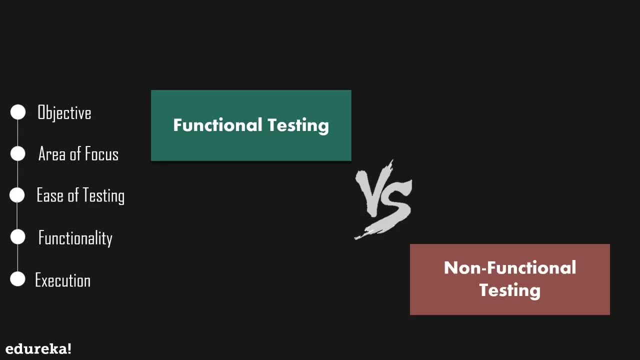 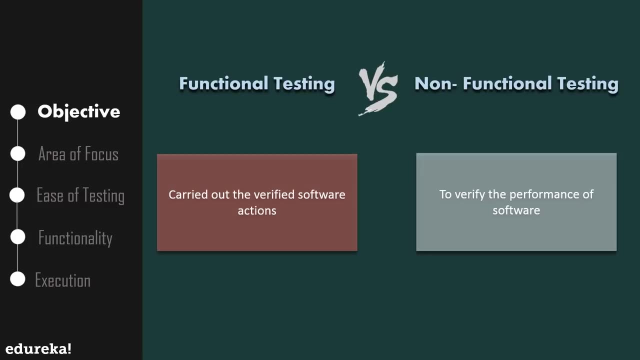 So we will have a look at the parameters, such as the objective, area of focus, ease of testing, functionality and execution. So the first parameter is the objective. now, in functional testing, It is carried out in order to verify the software actions, Whereas in non-functional testing it is used to verify the performance of 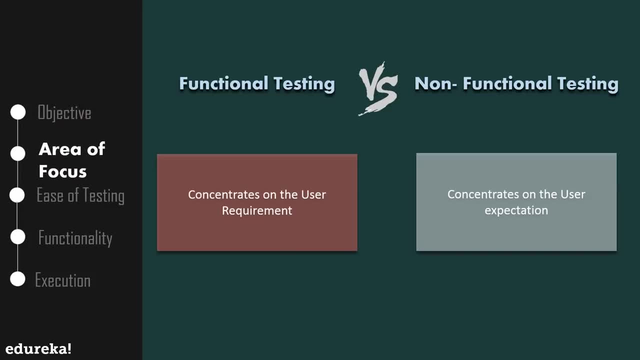 the software. next up is the area of focus. now, functional testing basically concentrates on the user requirement, whereas the non-functional testing concentrates mostly on the user expectation. the next parameter is ease of testing. now, functional testing is mostly used for black box testing, whereas non-functional testing is an easy way to execute the white box testing. 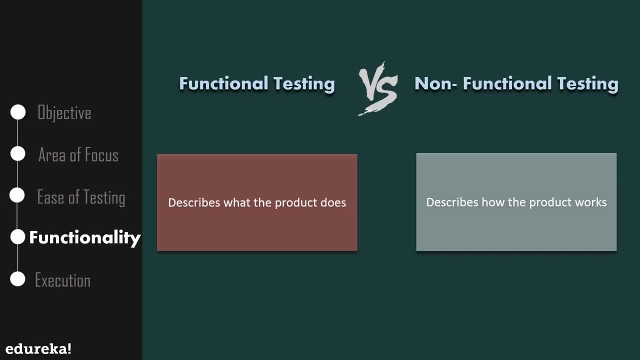 now, in case of functionality, the functional testing describes What the product does, whereas the non-functional testing describes how the product works. now, The final one is the execution. now, the functional testing always takes place before the non-functional testing, whereas the non-functional testing is performed right after the functional testing has been completed. 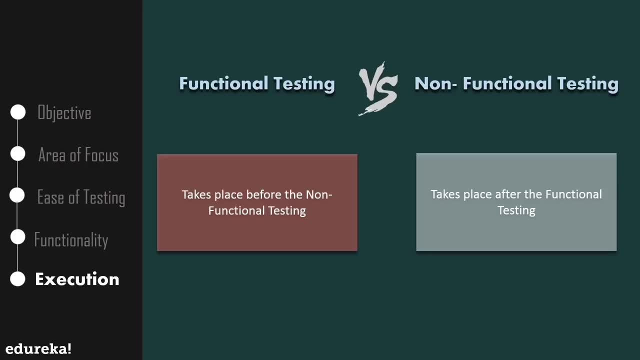 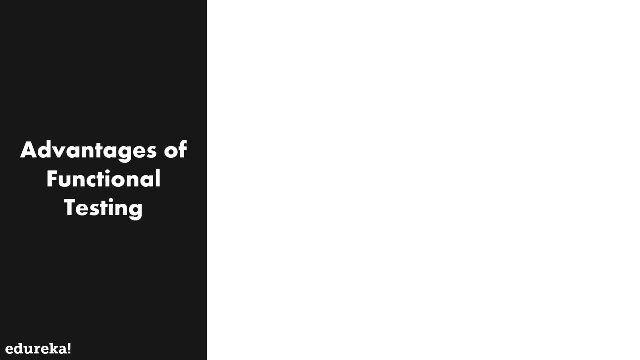 now, these were some of the differences between the functional testing and the non-functional testing. now let's have a look at some of the advantages of functional testing. that makes it more preferential. So this testing reproduces or is a replica of what the actual system is, that is, it is basically a replica. 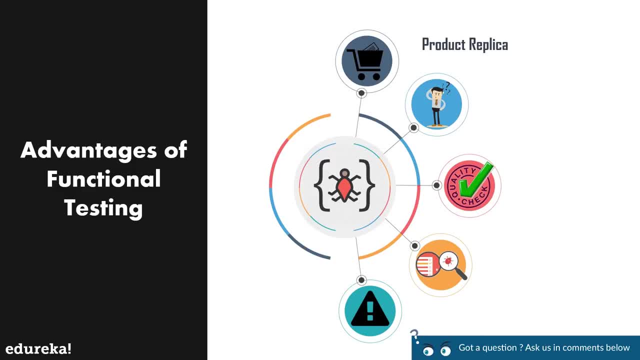 of what the product is in the live environment. now testing is focused on the specifications as per the customer usage, that is, system specifications, operating system, browsers, Etc. Also, it does not work on any if and buts or any assumptions about the structure of the system. 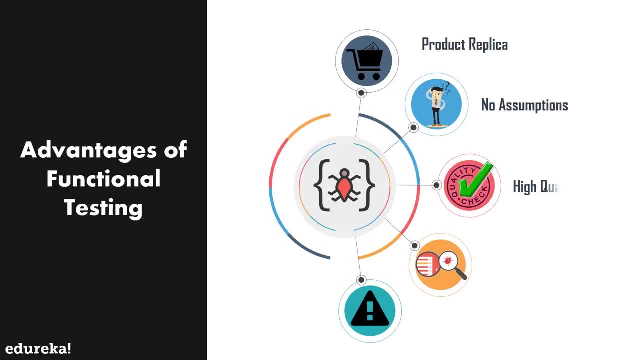 So basically, there are no assumptions for this testing next up. This testing also ensures to deliver a high quality product which meets the customer requirement and makes sure that the customer is satisfied with the end results. It also ensures to deliver a bug-free product which has all the functionalities working as per the customer requirement. 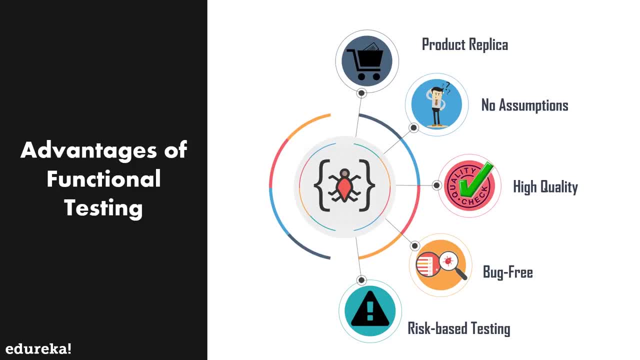 Finally, the risk-based testing is also done to decrease the chances of any kind of risk in the product. So now that we have seen all the advantages of functional testing, Let's move ahead and have a look at the different steps involved in this functional testing. 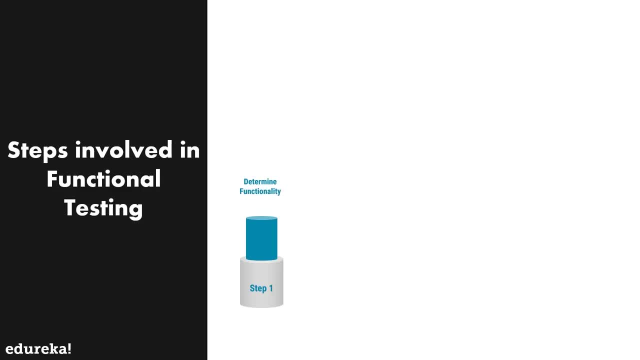 Now the very first step involved is to determine the functionality of the product that needs to be tested, and it includes testing the main functionalities: error condition and messages. usability testing, that is, whether the product is user-friendly or not. Now the next step is to create the input data. 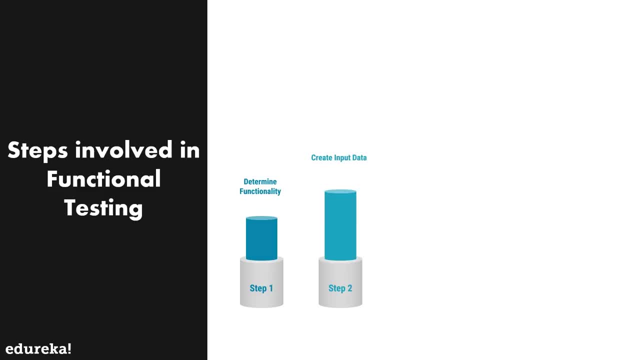 for the functionality to be tested as per the requirements Specification. later, from the requirement specification, The output is determined for the functionality under test. This is the step 3. here Now in the step 4, the prepared test cases are executed. and finally the actual output. that is the output after executing the test case. 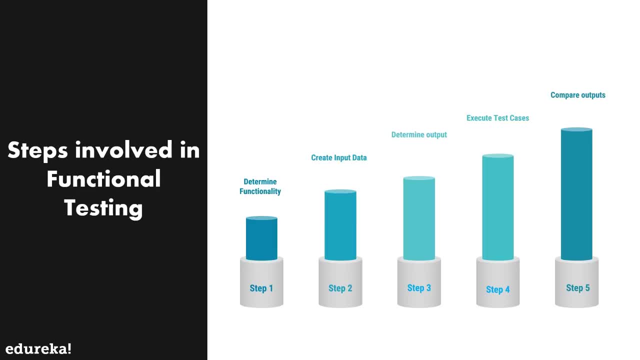 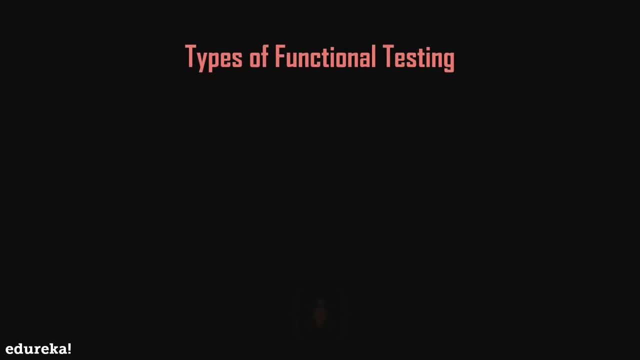 and expected output are compared to find whether the functionality is working as expected or not. Now, functional testing has many categories, and these can be used based on the scenario. So let's have a look at some of the most prominent types of functional testing. first up, 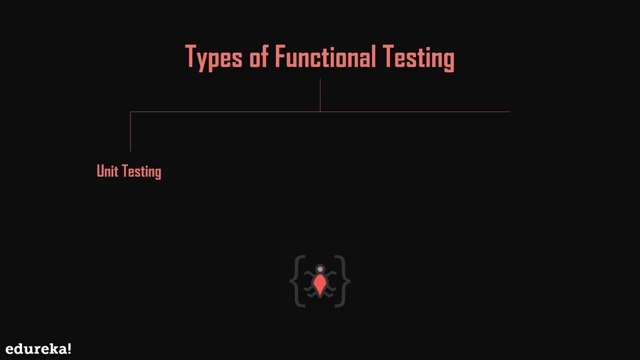 We have the unit testing now. unit testing is usually performed by a developer who writes different code units that could be related or unrelated to achieve a particular functionality. This usually entails writing unit tests, which would call the methods in each unit and validate those when the required parameters are passed. 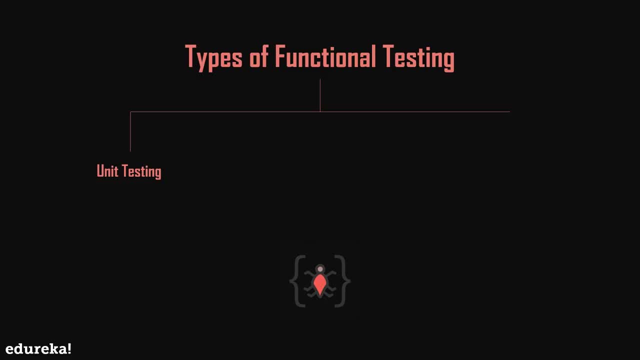 and its return value is as expected. now, code coverage is an important part of unit testing, where the test cases need to exist to cover the line coverage, code path coverage and the method coverage. next up We have the sanity testing. now testing that is done to ensure that all the major and vital functionalities 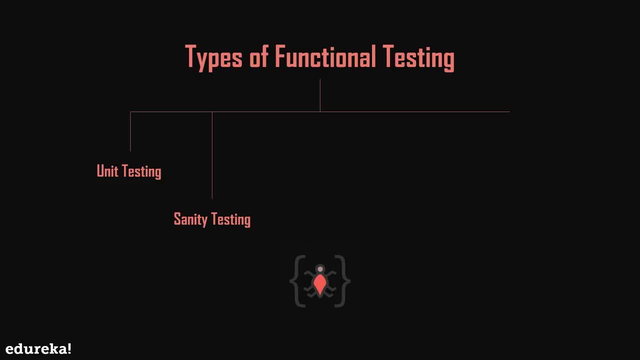 of the application or system are working correctly. Now this is generally done after a smoke test. So what is smoke testing now? the testing that is done after each build is released to test in order to ensure build stability is known as the smoke testing. it is also called 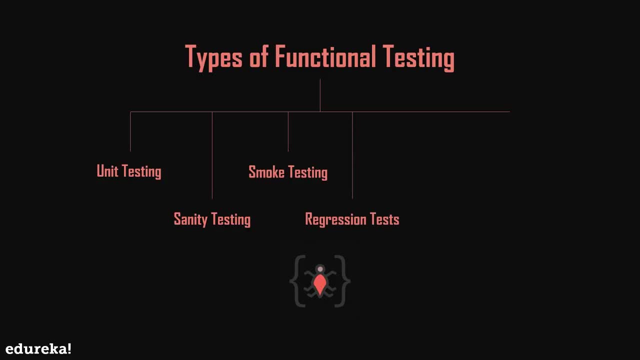 as build verification testing. then we have the regression tests. now testing performed to ensure that adding new code, enhancements, fixing of bugs is not breaking the existing functionality or causing any instability and still works according to the specifications. is known as the regression test. now regression tests and not be as extensive as the actual functional tests. 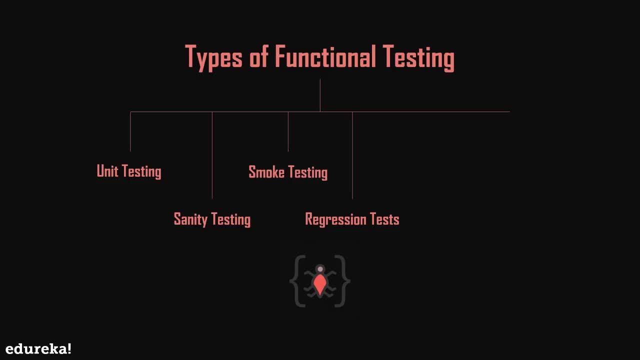 But it should ensure just the amount of coverage to certify that the functionality is stable. next up is the integration tests now, when the system relies on multiple functional modules that might individually work perfectly, but have to work coherently when clubbed together to achieve an end-to-end scenario validation. 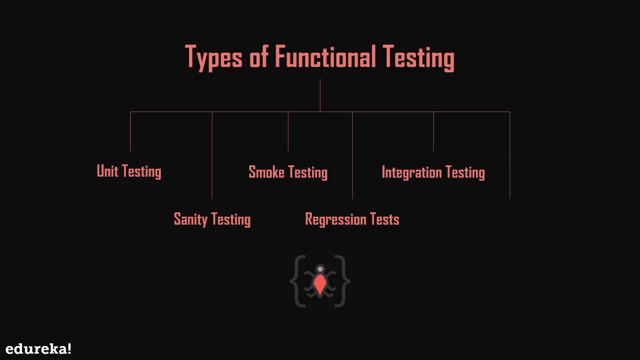 of such scenarios is called integration testing, and the final one is the usability testing. now The product is exposed to the actual customer in a production like an environment, And they test the product. the user's comfort is derived from this and the feedback is taken. 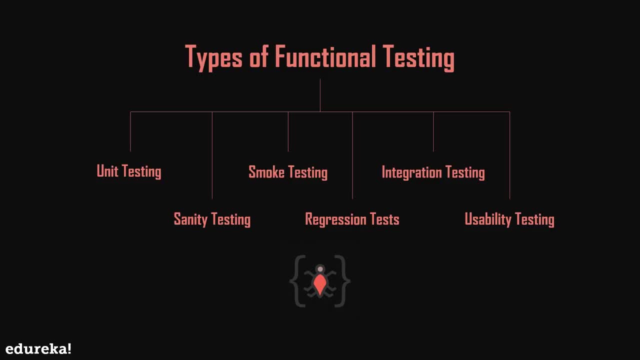 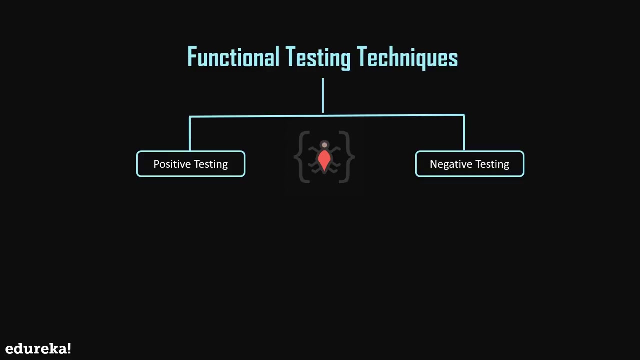 This is similar to that of user acceptance testing. So these were some of the important types of functional testing. now, moving on, Let's have a look at the different functional testing techniques. So, basically, we have two main techniques that are known as the positive testing and negative testing. now 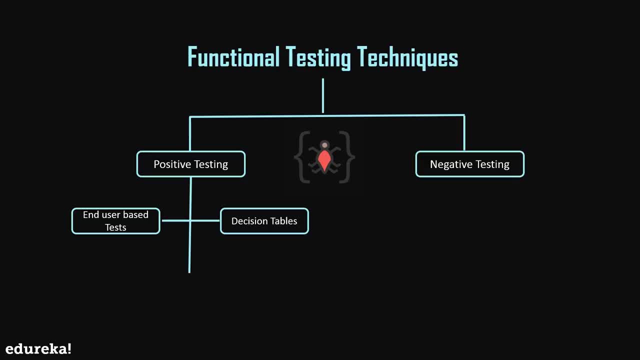 in positive testing. We have the end user based or the system tests. now, the system Under test may have many components which, when coupled together, achieve the user scenario. then we have the decision-based tests. now the decision-based tests are centered around the ideology of the possible outcomes of the system. 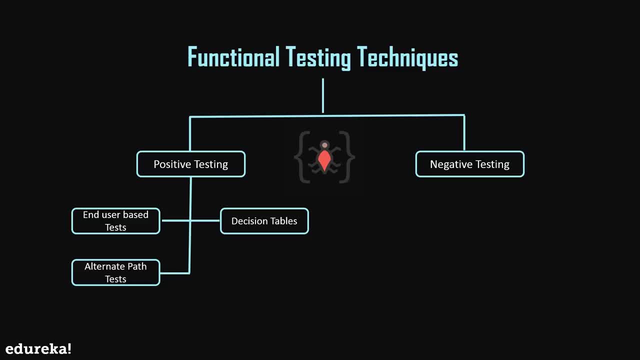 when a particular condition is met and the alternate flow tests are basically run to validate all the possible ways that exist other than the main float accomplish a function. now in negative testing We have the equivalence test. Now in equivalence partitioning, the test data are segregated. 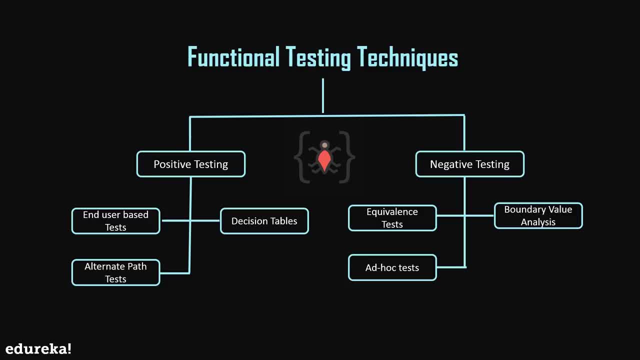 into various partitions, called the equivalence data classes. now, data in each partition must behave in the same way. Therefore, only one condition needs to be tested. Then we have the boundary value tests. now the boundary tests imply data limits to the application and validate how it behaves. 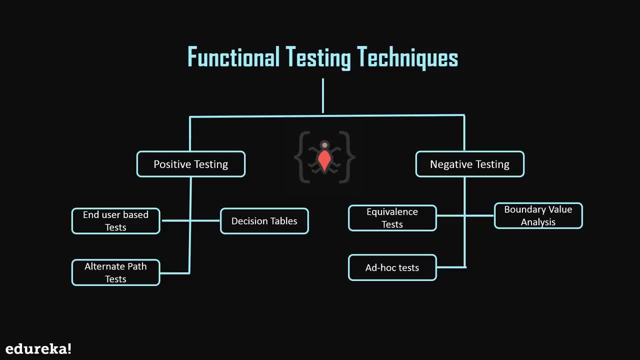 Therefore, if the inputs are supplied beyond the boundary values, then it is considered to be a negative testing. So a minimum of six characters for the user sets the boundary limit. Then we have the ad-hoc tests now when most of the bugs are uncovered. 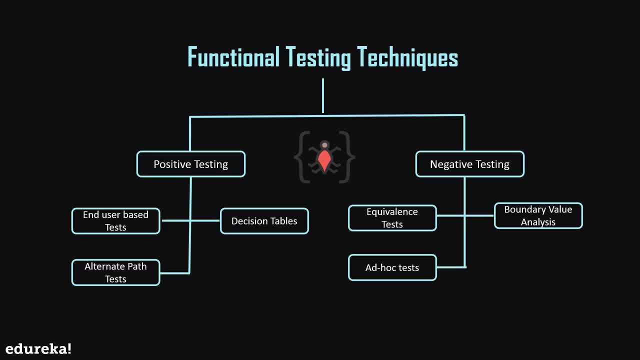 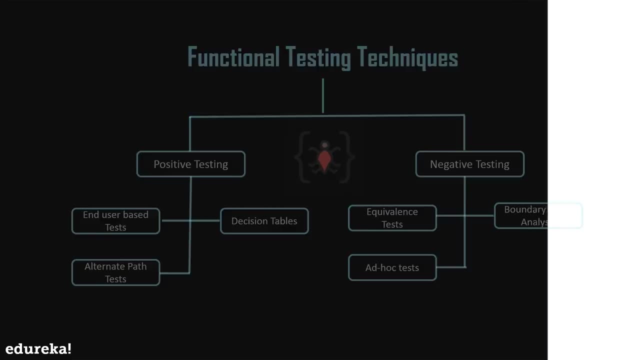 through the above techniques. ad-hoc tests are a great way to uncover any discrepancies that are not observed earlier Now. these are performed with the mindset of breaking the system and see if it responds gracefully. So these were the different techniques involved in functional testing. now, 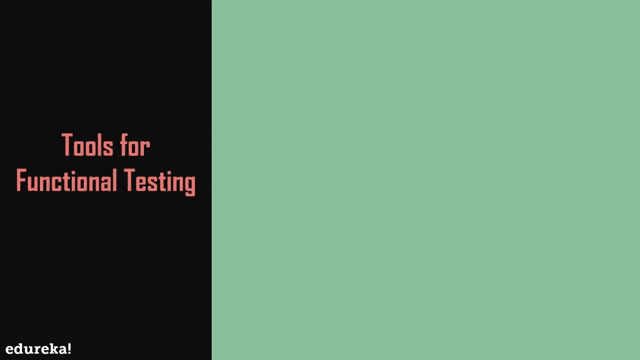 let's move on and have a look at the various tools that are used for this particular testing. now you can explore the best tool based on your project requirements. Almost every high-level company is working on automation in today's world, So just being a manual tester will affect one's career. 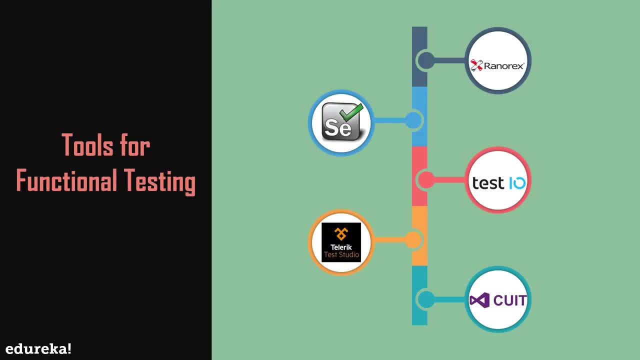 for sure. So you need to know something called automation to boost your skill and get shortlisted for some good companies. So now is the right time to know more about the need for functional testing tools, but which tools we should opt is really a confusing one. 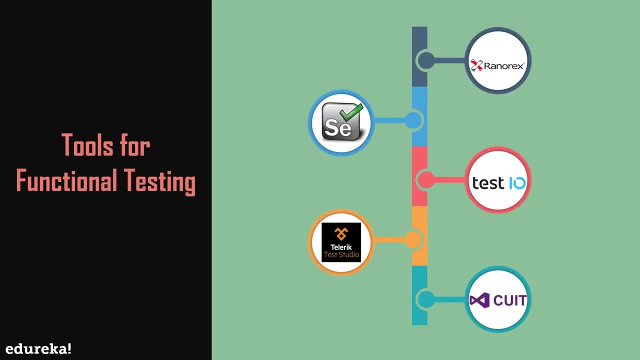 So let's have a look at some of the top most functional testing tools. So first we have the Ranarik studio. Now this one is a commercial Windows GUI test automation tool that supports functional UI testing on desktop, web and mobile applications. It is used by over 4,000 companies worldwide. 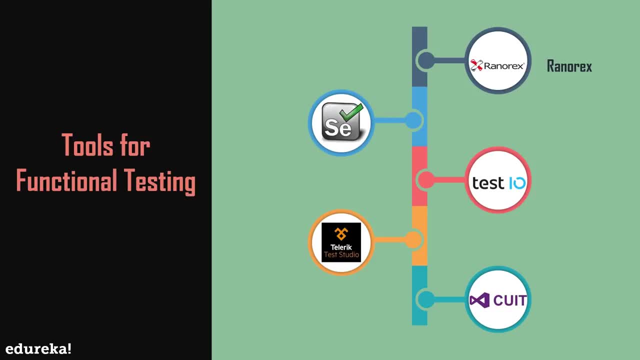 Now Ranarik studio is easy for beginners with a codeless click-and-go interface and helpful wizards, but powerful for automation experts with a full IDE. Next up, we have selenium. now selenium is an open-source functional testing tool, and one can download and use it without any cost. 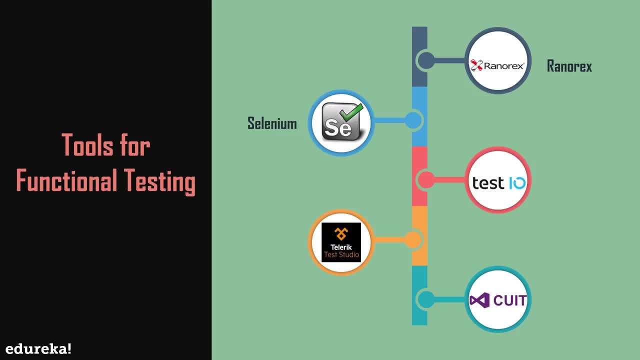 It is supported by the Apache 2.0 license. It is a web application testing product and it accepts many languages to write its test scripts and the languages can be C, sharp, Java, Pearl, PHP, Python, etc. It can be deployed on Windows, Mac OS and Linux. 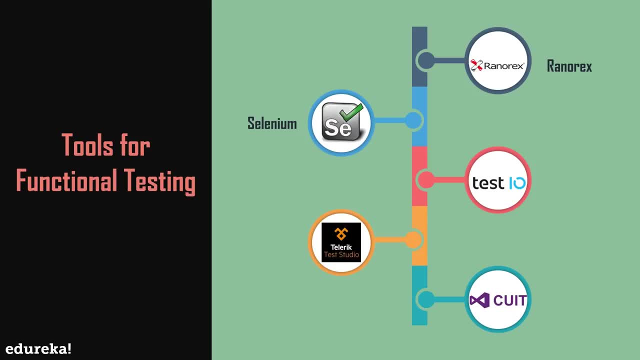 Now, this one is also one of the most preferable tools for functional testing. Now moving on next up, We have the test IO now for this. make sure that your web apps, websites and mobile apps work everywhere by running functional tests on real devices, real browsers and under real-world conditions. now running functional tests. 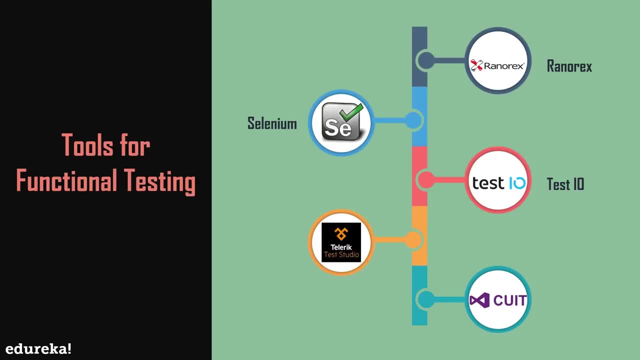 with test IO lets you call upon the skill and insight of thousands of testing professionals to improve the quality of your websites and mobile apps. over 200 customer obsessed organizations rely on the power and flexibility of test IO to ship high-quality software faster. Next up is the tell Rick now. 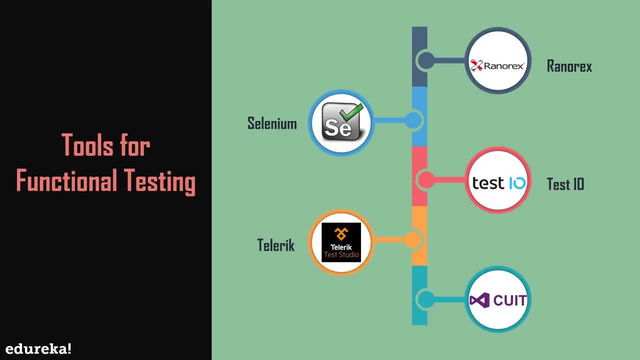 This is one of the most simple and user-friendly testing tools in the market. It provides functional exploratory performance as well as load testing solutions. though It's not free, its subscription to download the complete tool, along with its license, is available at a reasonable amount. 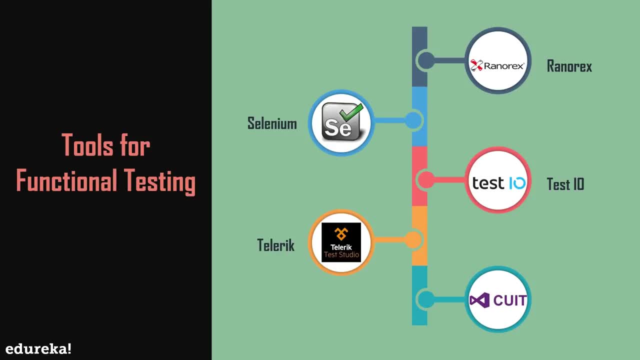 Now it comes with Visual Studio plugin. Hence, in order to bring the best out of this tool, one must know the visual script. Finally, we have the CUI test. now CUI test is a Microsoft tool. to use this tool, The user shall need Visual Studio 2013 virtual machine. 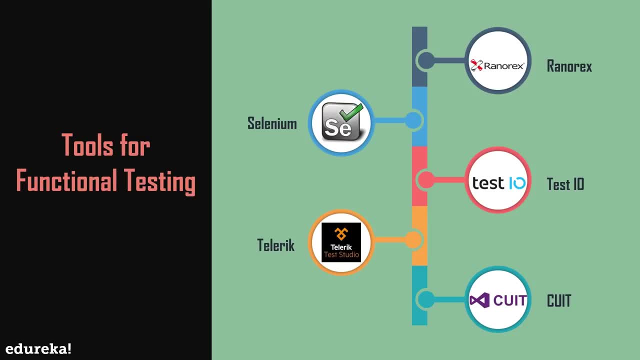 which is also a Microsoft product. now, by using the CUI test tool, one can completely automate tests for validating the functionality and the behavior of the application. now, before considering this tool, one must check for the latest cost of the CUI test tool and we STS license. 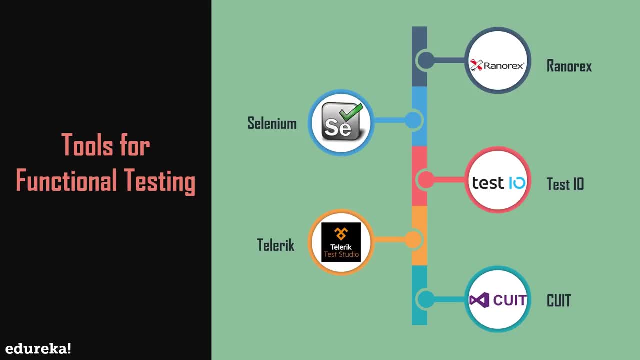 This cost with Microsoft? now, out of all these tools, selenium is one of the most preferred tools when it comes to functional testing, So let's have a look. what makes it the most preferable one? So let's talk about some of the advantages of selenium. 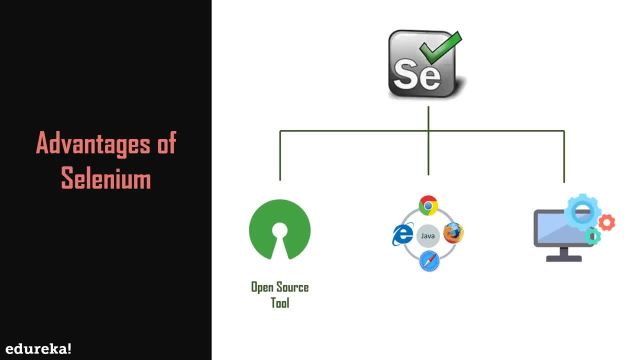 So selenium is basically an open-source tool which is used for automating the test cases carried out on web browsers or the web applications that are being tested using any web browser. So it's an open-source tool Which supports cross-browsing and automates web applications. 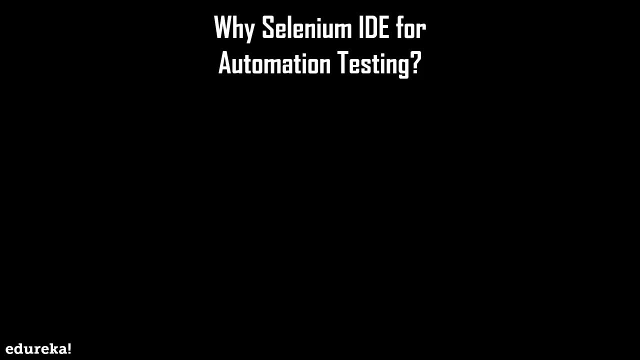 So now let's see why do we need selenium IDE for automation testing. now, selenium is basically an open source and also there is no licensing cost involved, which is a major advantage over other testing tools. Now, the other major reasons behind selenium's ever-growing popularity are about their test cases OS platform. 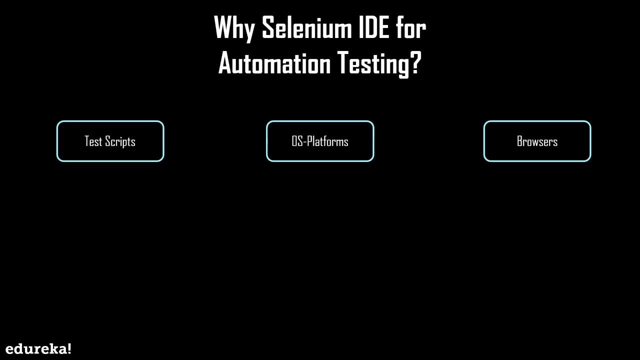 and browser support, So the test scripts can be written in any of these programming Languages, such as Java, Python, C, sharp, PHP, Ruby for and dotnet, and the tests can be carried out in any of these OS, such as the Windows, Mac or Linux. Also, the tests can be carried out using any browser. 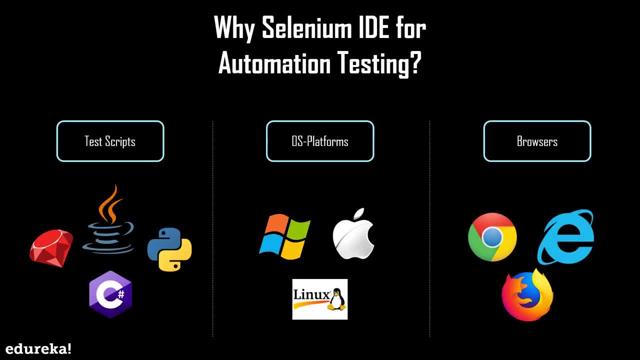 that is, the Mozilla Firefox, Internet Explorer, Google Chrome, Safari or Opera. So now that you know what is functional testing and also you have learnt about the best tool that is used for performing functional testing, Let's have a look at a small example that will help you understand. 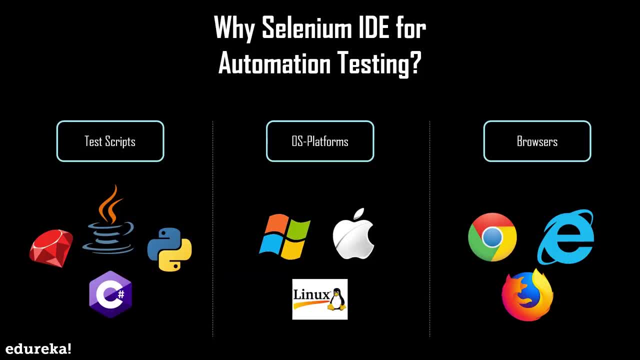 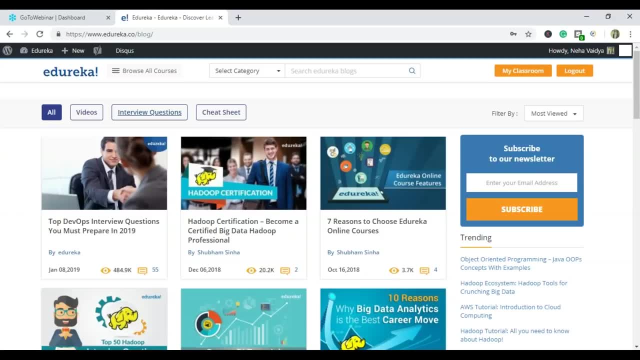 how we are performing this functional testing with the help of selenium. So now let's have a look at the example. So here we will be performing functional testing with the help of selenium. So let's take the example of our edureka blog page. 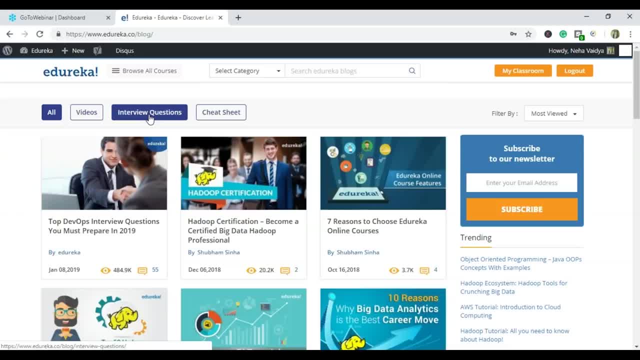 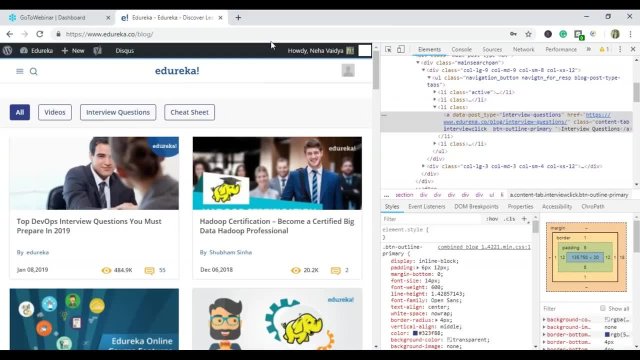 So now, if I want to click this particular element, let's see how I can do this with the help of selenium. So now this can be done with the help of locators. So first let's see what are locators in selenium. 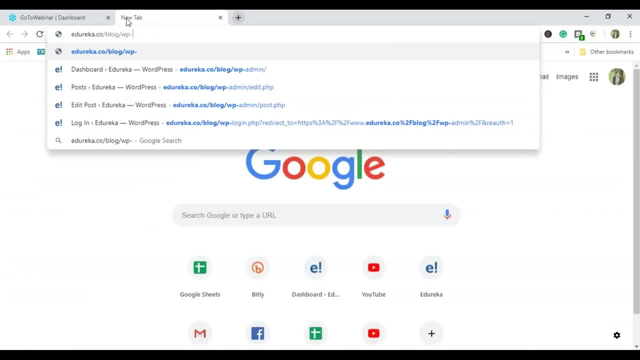 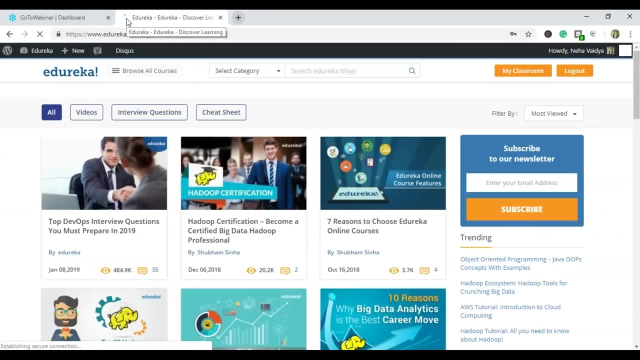 Now the locator can be termed as an address that identifies a web element uniquely within the web page. Now locators are basically the HTML properties of a web element, which tells selenium about the web element It needs to perform the action on selenium users locators- to interact. 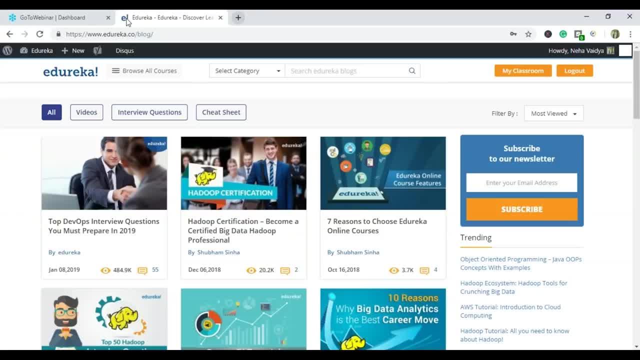 with the web elements on the web page. Now there is a diverse range of web elements, like the text box, ID, radio button, Etc. Identifying these elements has always been a very tricky subject, and thus it requires an accurate and effective approach thereby. 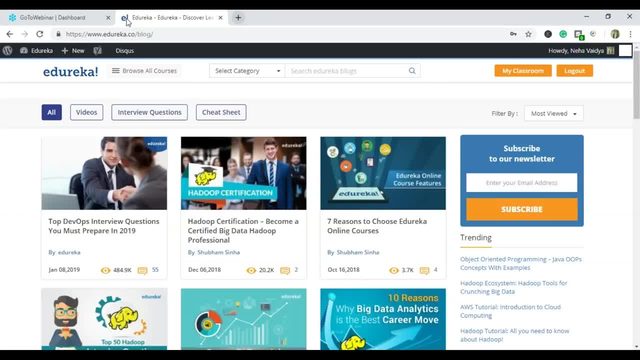 We can say that more effective the locator is more stable will be the automation script. essentially, every selenium command requires locators to find the web elements does to identify these web elements accurately and precisely. we have different types of locators, namely the ID name link text, CSS. 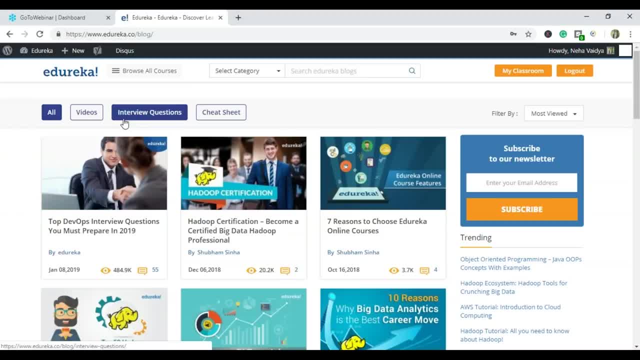 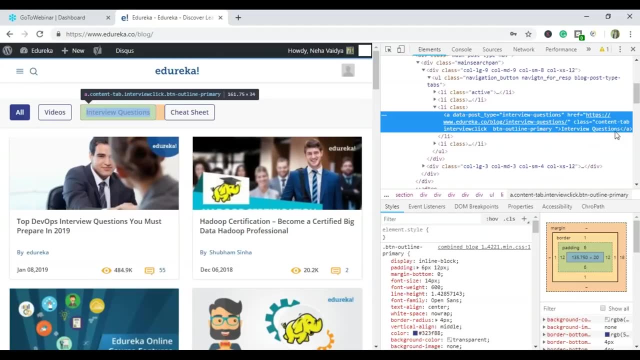 Select a partial link text and XPath. So now, in this particular case, I'm using the link text to connect to the particular link. So here we will be clicking on the interview questions and select on inspect. now here We will get to see a link text named as the interview questions. 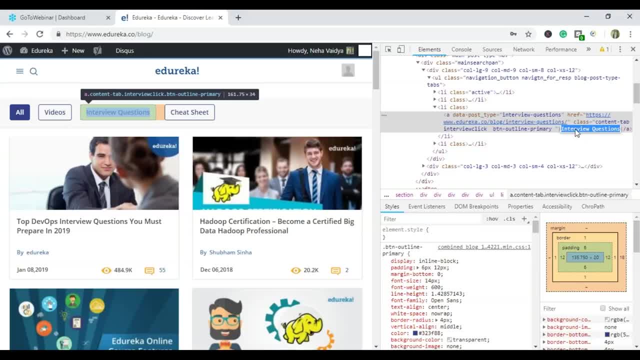 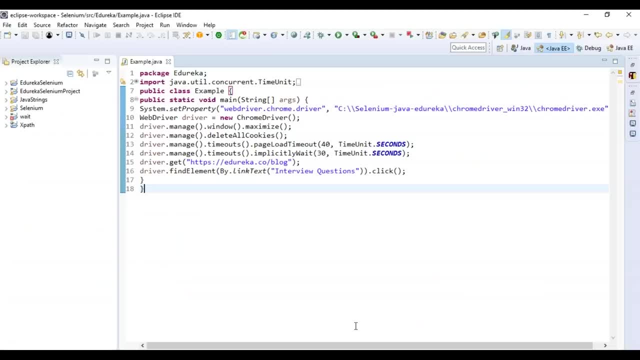 So here I'll copy this and use the link text locator to locate the element. Now, before that, let me first tell you what is link text. now all the hyperlinks on a web page can be identified using link text. Now the links on a web page can be determined. 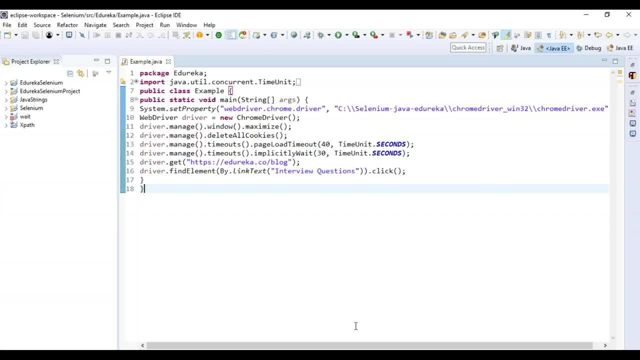 with the help of anchor tag. Now, the anchor tag is used to create the hyperlinks on a web page, and the text between the opening and closing of anchor tags constitutes the link text. So let's switch back and see how we are going to do it. 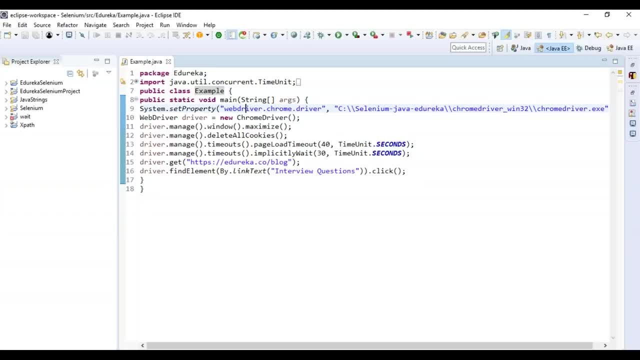 Now this is the example that we are going to use for our test. So first of all, I have created a class named example and after that I have set the property Where I have used the Chrome driver and, next up, I have used the systemset property.